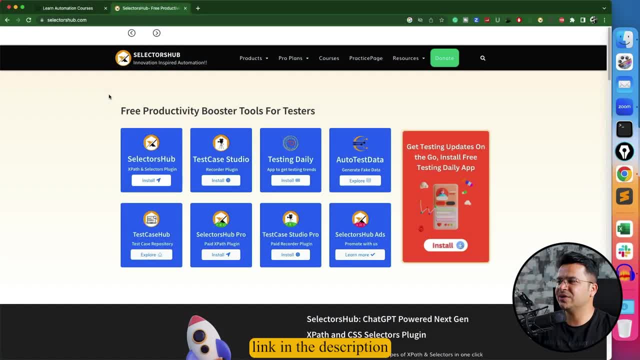 tools and so on. so let me show you how you can use it. so let's navigate to selectorshubcom. so this is by Sanjay Kumar. so, first of all, thank you so much, Sanjay, for these amazing tools. all these tools- selectorshub, testcase, studio testing, daily autotest data- all tools are amazing. obviously they 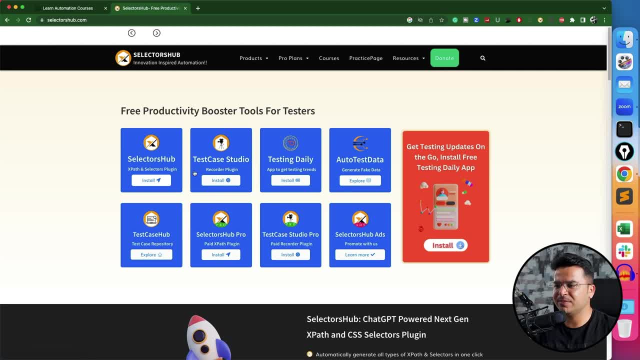 have some pro versions. that is orthodot and they have all the information that is in there. we just that is additional part, but all these are for the community. so today that we are going to talk about is test case studio, which can help you to generate the manual test cases and steps to do produce. so 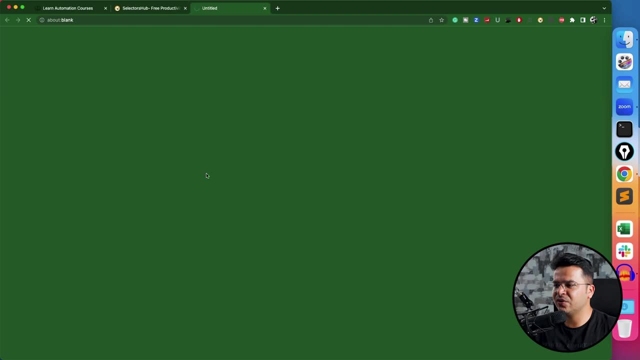 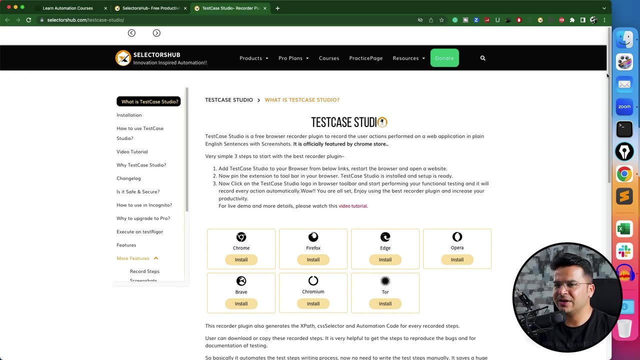 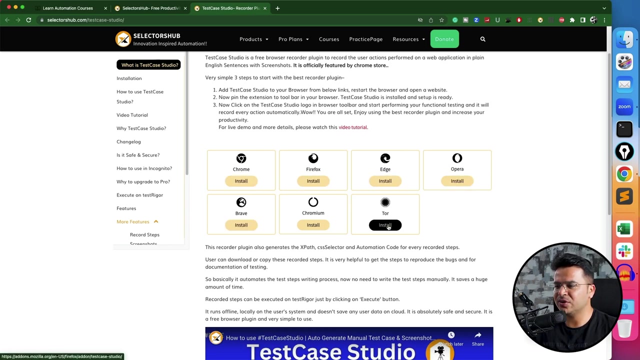 you can navigate to selectorshubcom and just go to test case studio. now you can directly go to the chrome store and you can do that as well. it's totally up to you, and right now this plugin is available for all the popular browsers so you can see chrome, firefox edge opera. brave chromium tor. 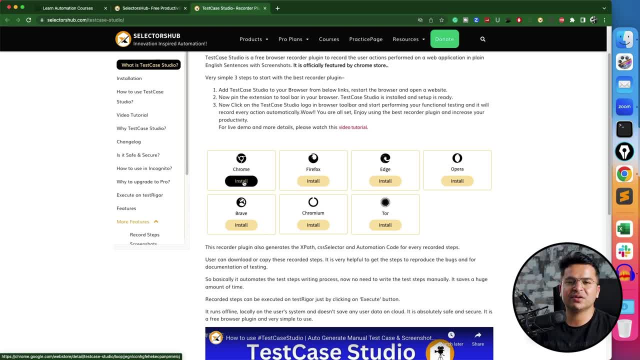 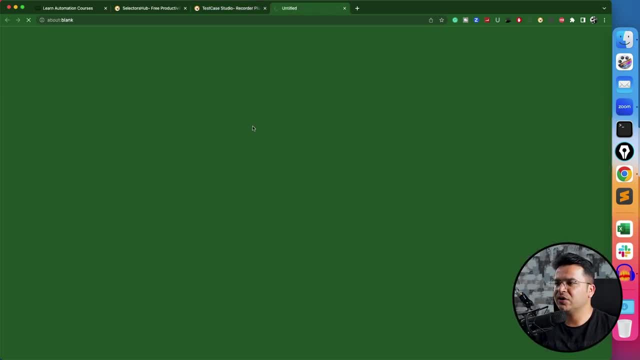 so let's continue with chrome. i'm using chrome, but feel free to use this with any other browser. if you face an issue, let me know directly or you can connect with sanjay as well. the moment you click on install, it will ask you to install this plugin again. it's a safe plugin, don't worry about. 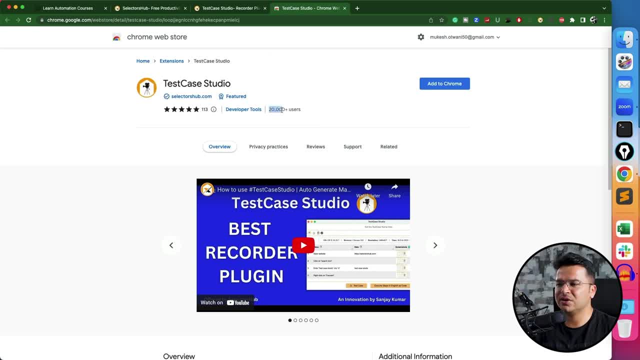 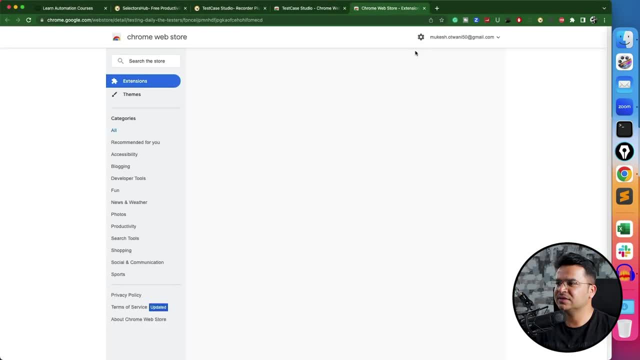 it and if you see the five star rating, more than 20 000 users are already using. so let me click on add to chrome and add extension and it says this extension has been added. yes, you can see that it has been added. so let me click on add to chrome and it says this extension has been. 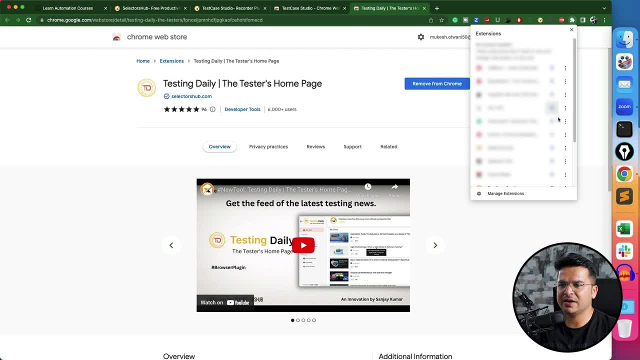 added. so let me click on add to chrome and it says this extension has been added. yes, now this extension will not show you directly. you have to click here and scroll down. you will find test case studio. so let me pin this and here is the test case studio: how to use it. now i'm using 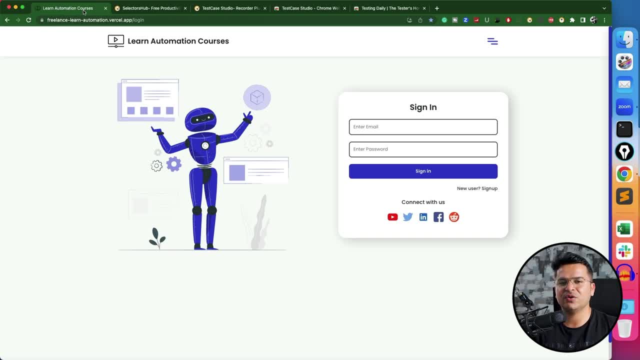 one sample application, but feel free to use any application. you have to use your own application and generate the manual test cases. so once this is done, let's say i want to write manual test cases for this application. so what i will do? first of all, i will just give you some idea about this. 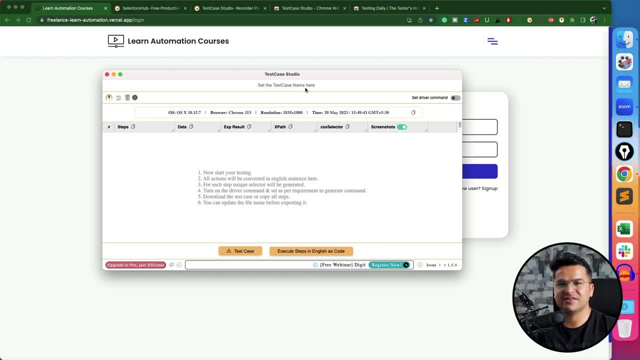 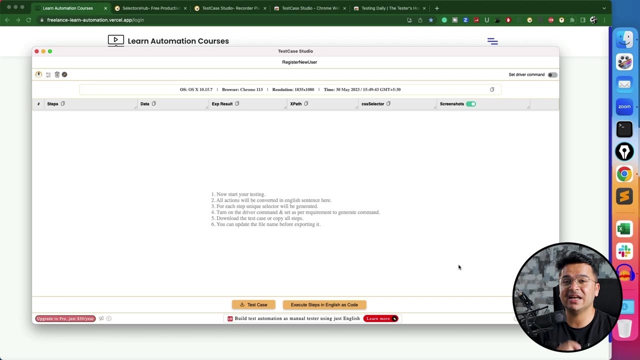 particular plugin. so, first of all, you can set the test case name here. in my case, let me write this: register- new user. this is the test case name that i have added. the very important feature which i found is the screenshot. it can generate the screenshot for each and every step that you will be writing. 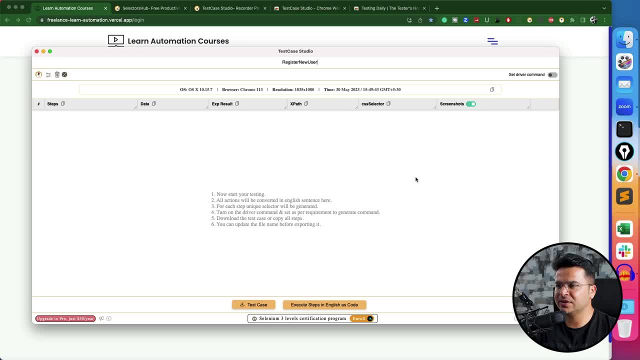 you can see all the details. it is showing which browser, using what resolution and the time. now let me show you this part. so this is the button. if you want to stop the recording, you can stop here. the moment i click on this plugin, it started the recording. so as of now, let me stop the recording. 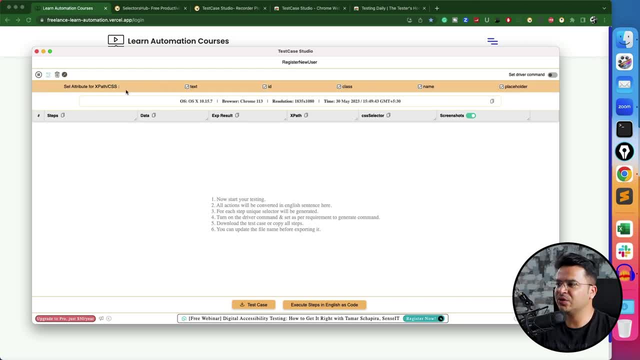 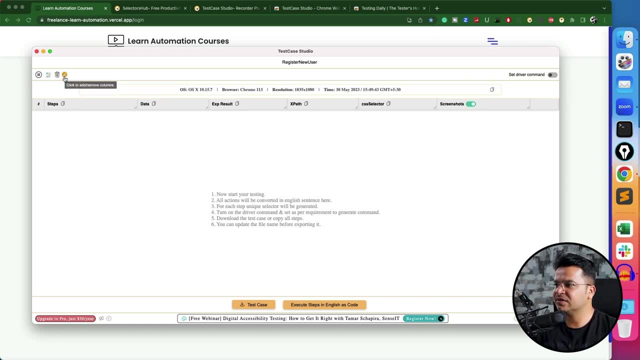 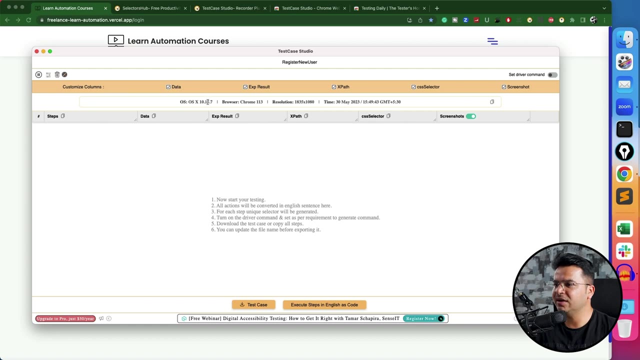 first of all, and you can see in case, if you want to use some attribute for xpath and CSS, you can select and deselect from here and this is the most important part: click to add and remove column. so let's say, right now i can see six column, right, maybe i don't want xpath for writing the test cases. 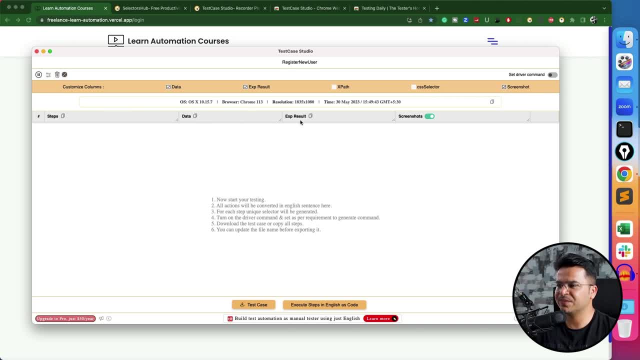 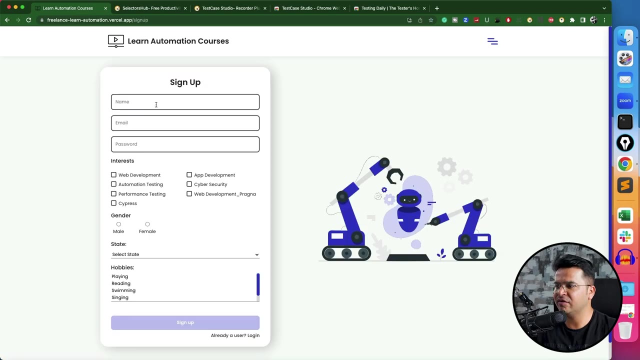 maybe i don't want css steps, data, expected result and the screenshot and we are good to go. so now, if you click on click to start recording, recording is on already and this is my web application. let's say I want to create a new user and I will be lending. 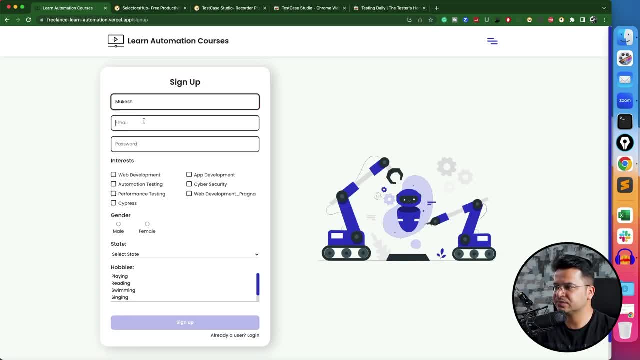 to this page. now I will continue here. let me write the email address part now. notice here it is highlighting as well. okay, so let me quickly fill this page. automation testing mail select state. let's say. go up, it's highlighting again and I prefer reading, so click on reading the moment. I click on sign apart and see. 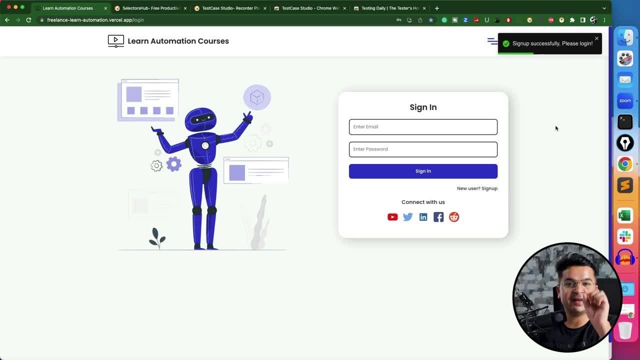 I clicked here and it highlighted as well. this is the very interesting part. sometimes even few elements will come for a hardly few seconds. even it is able to capture that as well. now, once it is done- let's say I want to see- I will click here once again. and now. 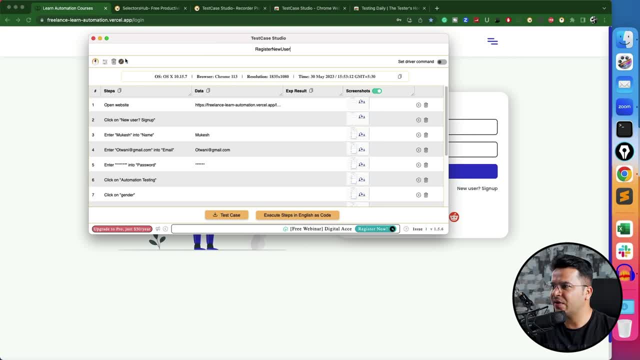 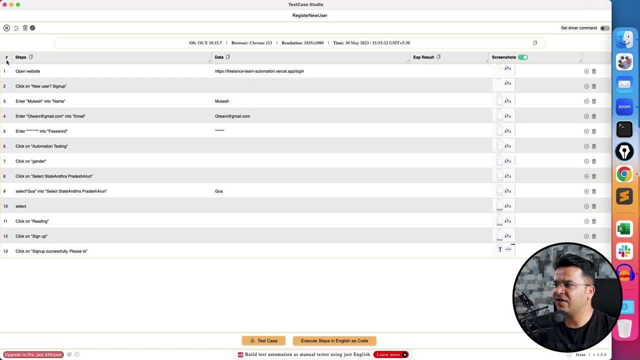 you can see I got all the steps here. now I can stop this recording and this is my test case ready. first of all, you can see it has identified. first one is the number of steps that I have performed, then the data, expected result screenshots: okay, one by one. open website. it opened the URL, then it clicked on new. 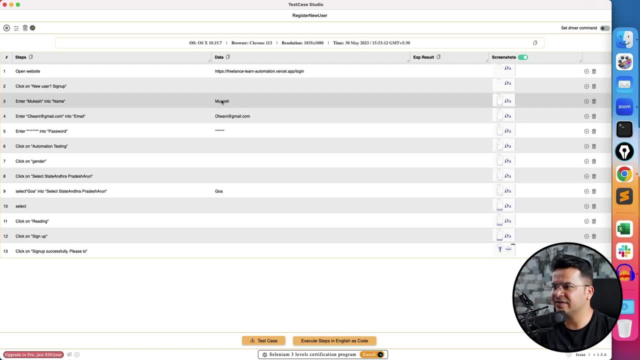 user sign up link: enter Mukesh and then click on start recording. this is the text data, right then again, this is the email, and good part is it is masking the password. okay, so whatever password I have entered, it is already showing in a mask. then click, click, click, click, select, click and finally, right now. 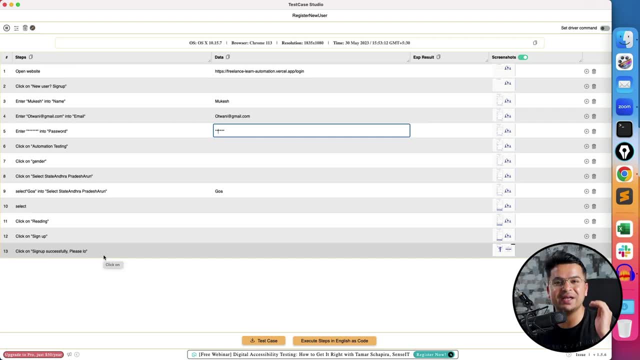 in this application. I did not perform any scrolling, but if you have a scrolling, it can do the scrolling record as well. perfect. so once you are done with the test cases, you can see this option called test case. the moment you click on this, it will start downloading the test case. okay, you don't need to copy. 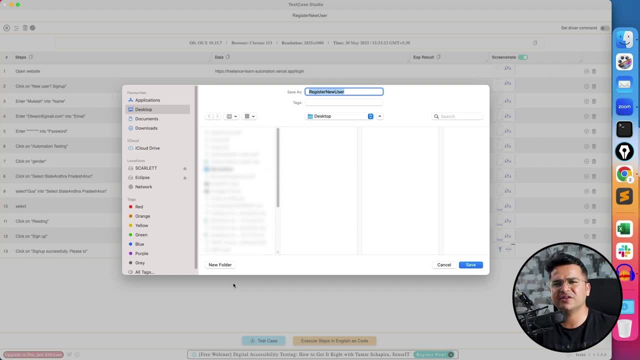 here you can download as Excel and then you can use this to any test management tool that you're using. okay, so, whether it's a Jira test trail or any other test management tool, you can simply copy paste this data and continue. so let me click on desktop. I want to save everything on the next top. now it will. 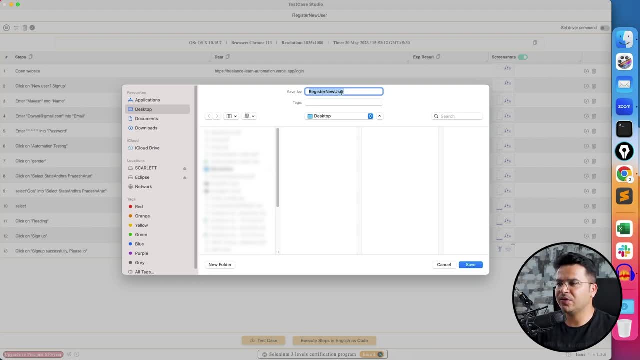 ask me in case if I want to rename, I can rename it right now. I want to keep register new user. click on save, so it already one. it has downloaded already one excel file, as you can see, dot XLS. now it is downloading one more folder for the screenshot. 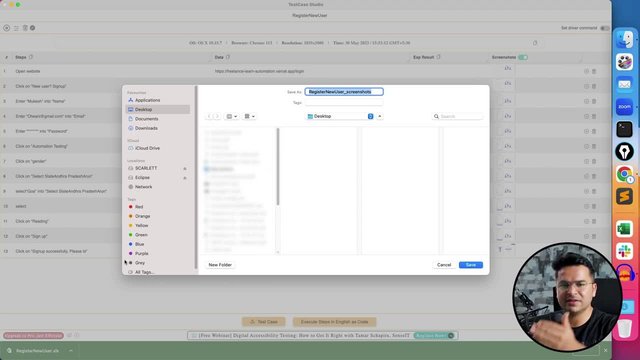 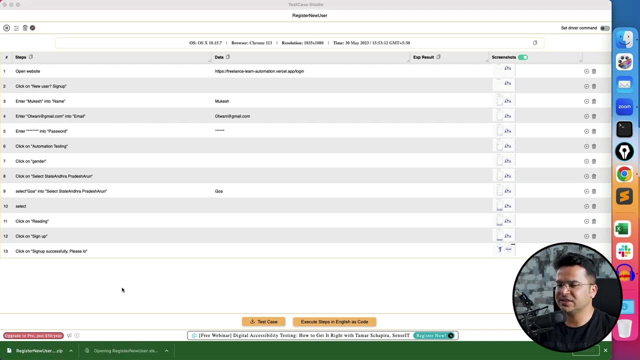 so that if you, whenever you want to use screenshot, you can directly take the screenshot and continue. so again, I will not change this. let me keep on the desktop again. so let's open this excel sheet once again and it will give you this alert. it says: do you want to open it? anyways, I will say yes and yes, my 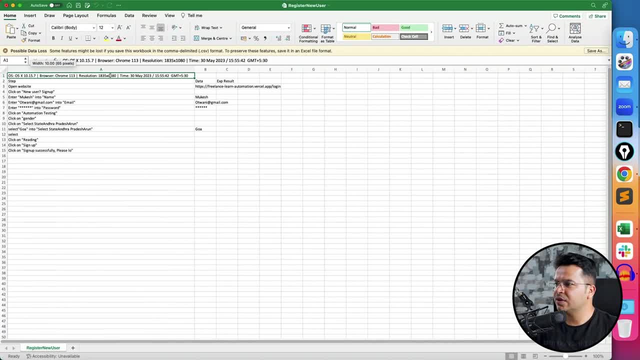 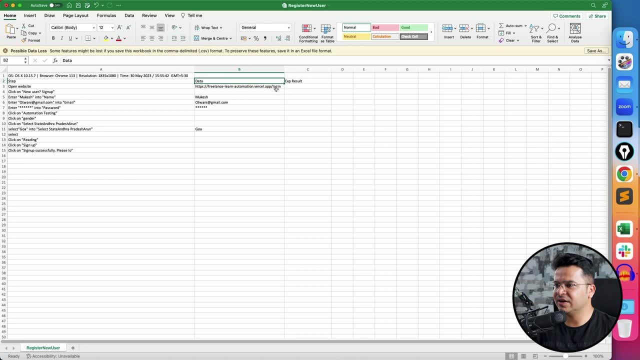 excel sheet is ready here now. whatever details you don't want, you can remove it. okay, so right now it has given you all the steps plus the test data and the result. you just need to add the actual result and you can start executing the test. right now I'm showing in Excel, so I'm manually adding this column, but let's 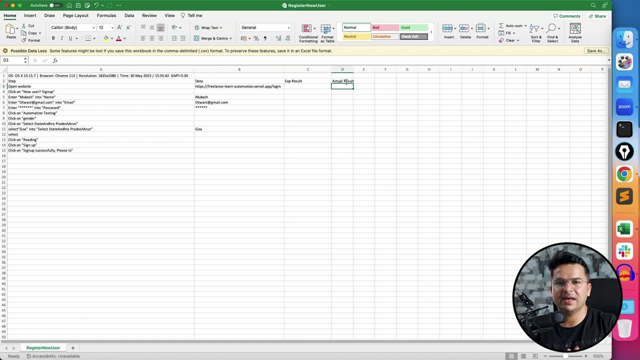 say, whenever you're using in test management tool, you will be getting the expected and actual results. you have to modify a few things from your site. what is actual result? what is expected? if it is mismatched, then you have to raise a book. now, if you do only want the steps, you can copy and you can continue right. 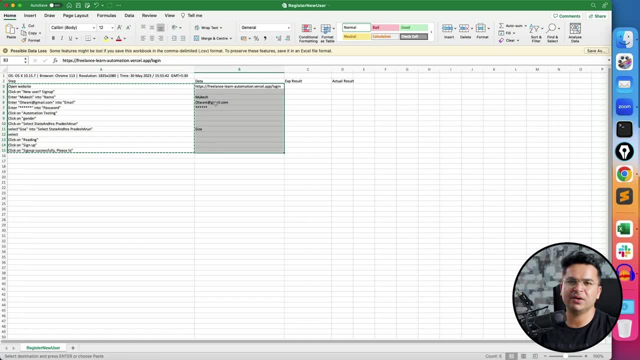 in case, if you want to change the test data, you can directly change from here or you can directly change once you start writing the test cases in the test management tool. so this is one of the most important part which I wanted to show you. another interesting part is this zip file that we will be getting, so